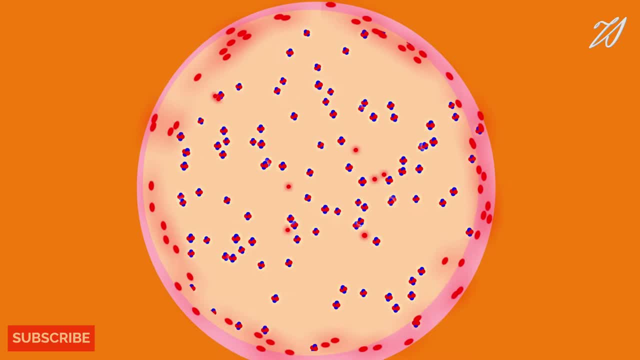 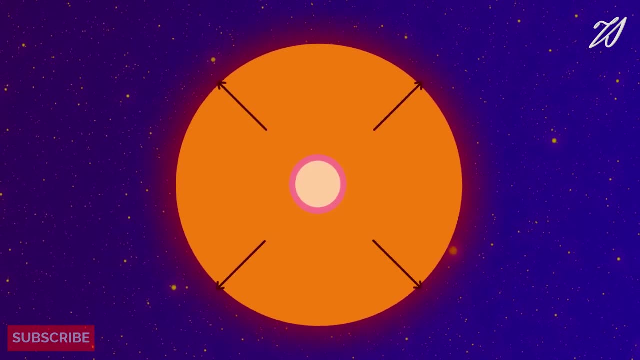 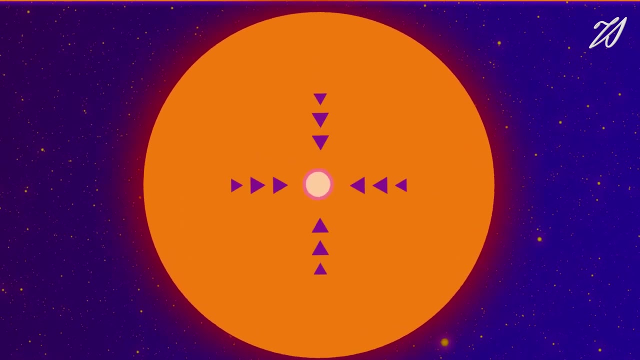 As helium is denser than hydrogen, the remaining hydrogen moves towards the outer core and envelops the core. The star swells up. At this stage, the temperature of the core won't be sufficient enough to fuse the helium accumulated in the core. 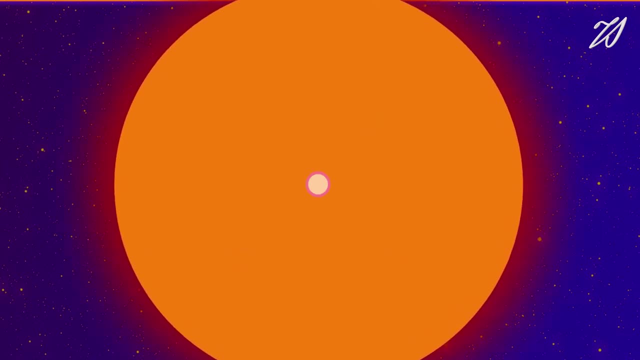 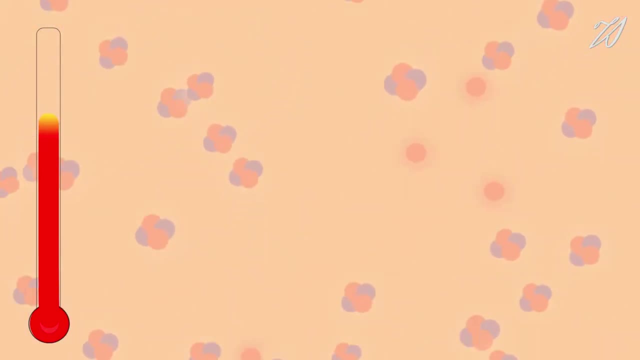 The core contracts due to the gravity acting towards the center of the star. As the core keeps on contracting, the temperature of the core increases. When it reaches 100 million Kelvin, this center of the core will be at the center of the core. 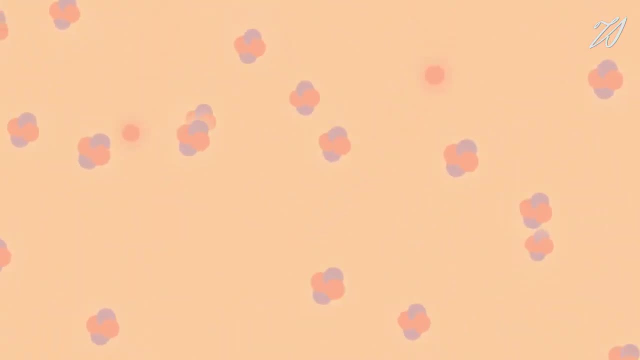 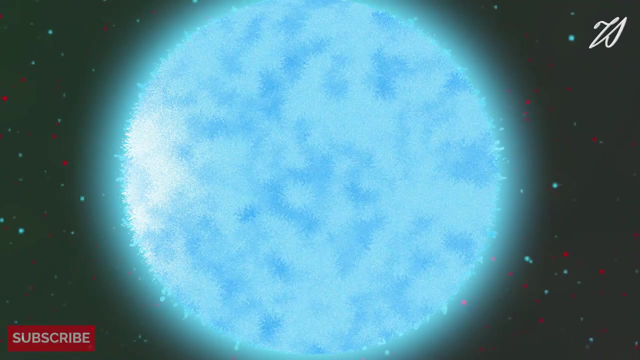 The sub-giant phase of the star ends and helium starts fusing to form carbon. Supermassive stars jumpstart the helium fusion quickly. At this stage of the stellar evolution, the star becomes a red giant or, if it is a massive star, it becomes a supergiant. Thus, in each stage, the star will fuse heavier atoms to make much heavier atoms. This nuclear fusion continues until the stellar core fuses. The nuclear fusion continues until the stellar core fuses. This nuclear fusion continues until the stellar core fuses. 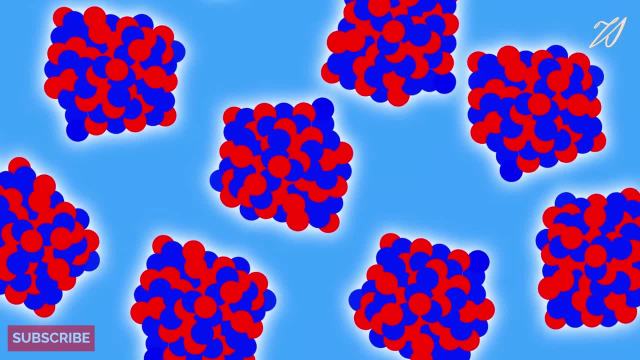 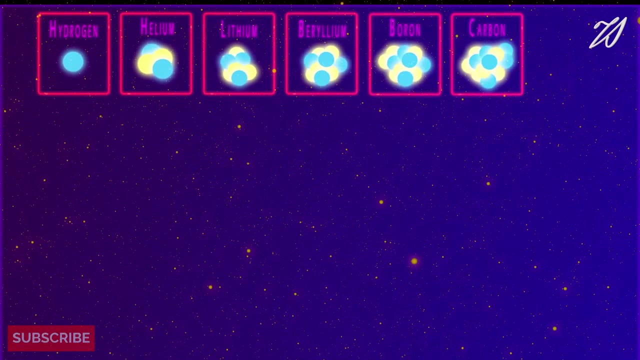 This nuclear fusion continues until et drosophila oxygen fills with iron. As iron is the most stable element, nuclear fusion reaction cannot proceed any further. If we look in the periodic table, all the elements up to iron are synthesized inside the stellar core. 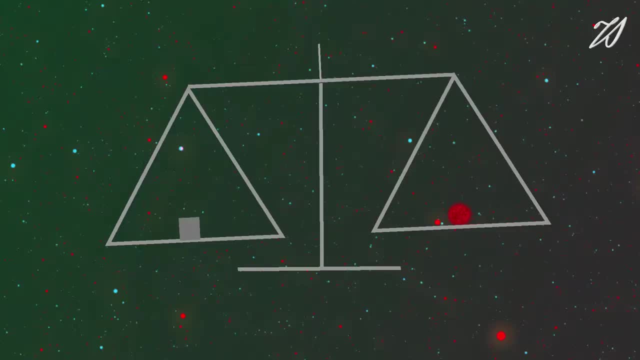 All stars won't fuses elements up to iron. How far a star fuses elements depends upon its mass. We can divide stars into three categories: The stars with mass less than Like the stars, Kubernetes and the sort of stars that gamma spare to use. 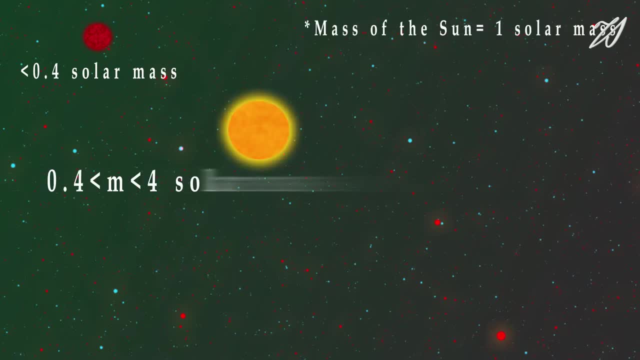 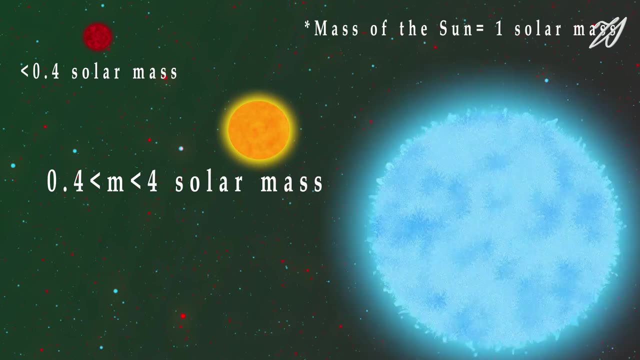 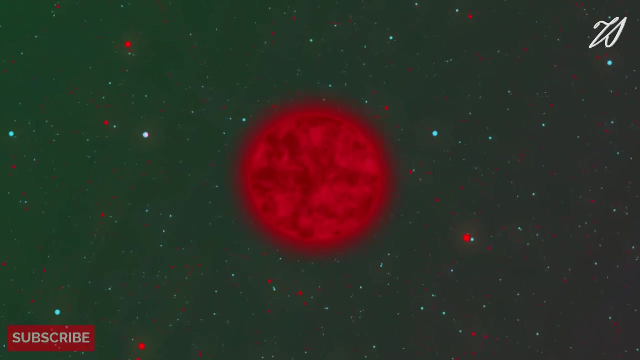 less than 0.4 times the mass of the Sun. the stars whose mass lies between 0.4 and 4 solar mass. it includes our Sun. and, finally, massive stars with mass greater than 4 solar mass. those stars with mass less than 0.4 solar mass is too cool to. 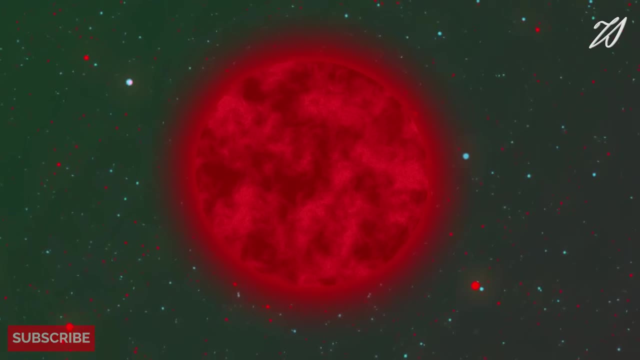 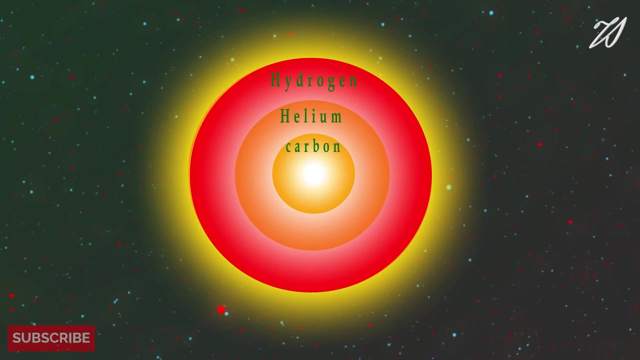 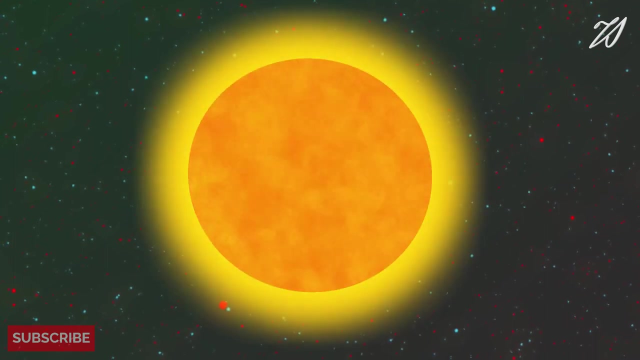 fuse helium. once it completes the hydrogen fusion, it ejects the hydrogen shell into space and becomes a white dwarf made of helium. stars with mass lying between 0.4 and 4 times the solar mass will fuse all the way up to carbon and oxygen. it cannot fuse to further, heavier elements. those stars end up as